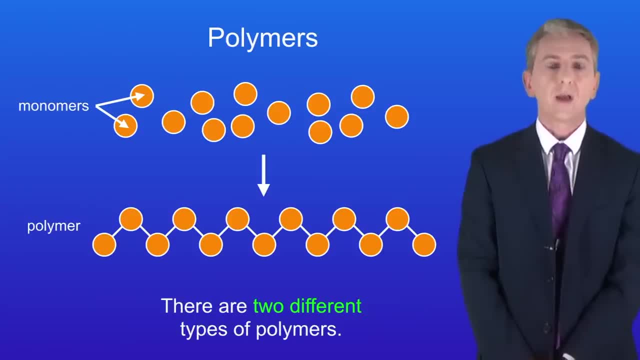 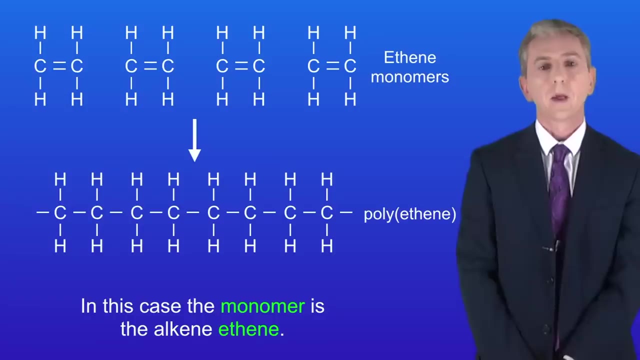 polymer. Now, there are two different types of polymers. These are called addition polymers and condensation polymers. In this video, we're looking at addition polymers In addition polymers. the monomers are alkenes and in this case, the monomer is the alkene ethene. We've joined the 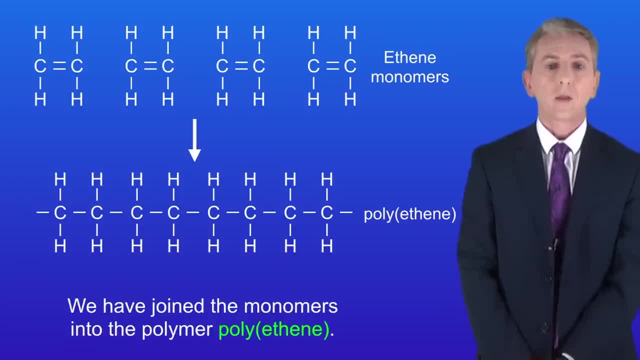 monomers into the polymer polyethene. Now there are a couple of points about this. Firstly, the monomer has a double carbon to carbon bond, but the polymer has single carbon to carbon bonds. Secondly, the name of the polymer is the word poly, followed by the name of the monomer. 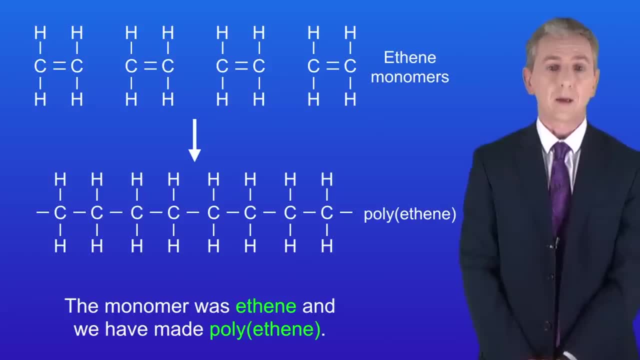 So the monomer was ethene and we've made poly ethene. The word poly simply means many. Now students sometimes ask what happens at the ends of the polymer, but at GCSE you're not required to know that. Okay, now scientists have a shorthand way of showing the structure of a 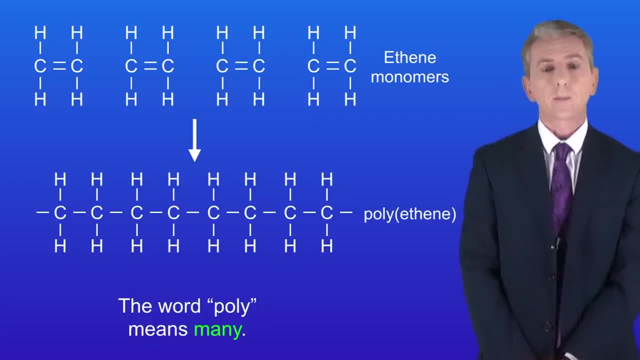 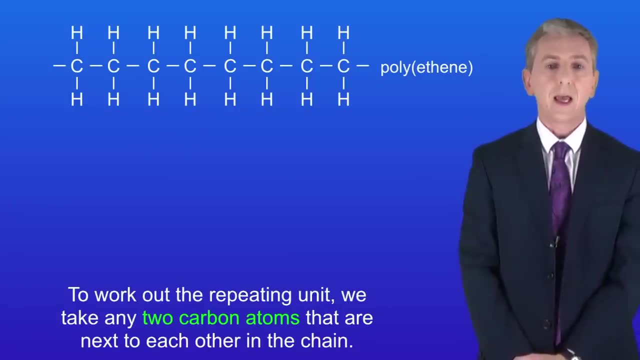 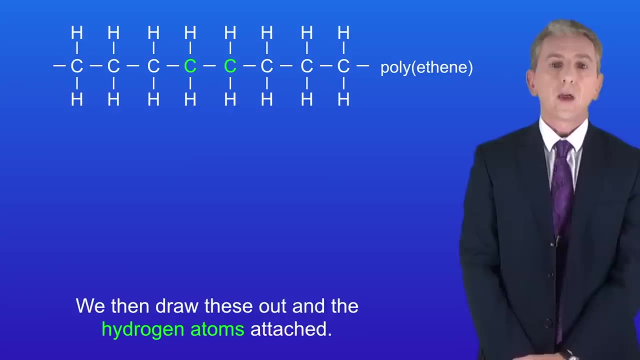 polymer and that's called the repeating unit. We're going to look at that now. I'm showing you here polyethene again. To work out the repeating unit, we simply take any two carbon atoms that are next to each other in the chain. I'm taking these two. 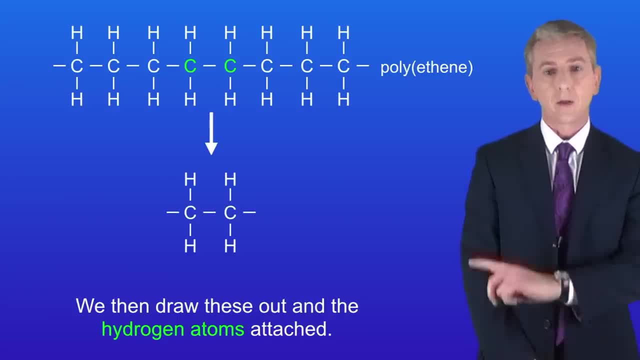 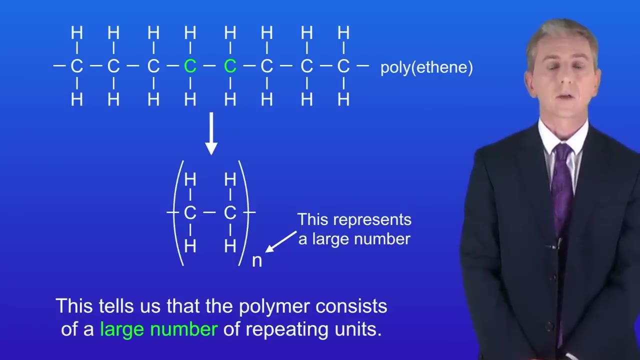 We then draw these out and the hydrogen atom is attached like this. Next we place brackets around them and finally we write a small n to the right. The n represents a large number. This tells us that the polymer consists of a large number of repeating units. Now I'm 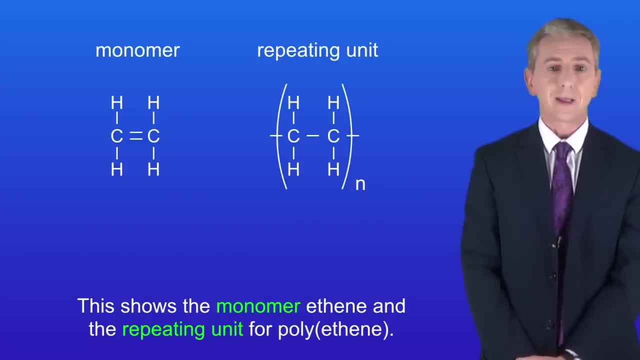 showing you here the monomer ethene and the repeating unit for polyethene. This brings us to a couple of important points. Firstly, in addition polymers, the repeating unit has the same atoms as the monomer. That's because no other molecule is formed in the reaction. 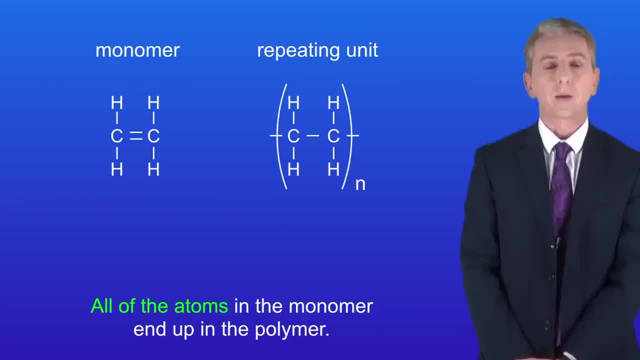 In other words, all of the atoms are the same. In other words, all of the atoms are the same in the monomer end up in the polymer. Secondly, remember that the repeating unit does not contain a double bond. Now in the exam, you could be asked to draw a polymer, given an alkene monomer. Here's: 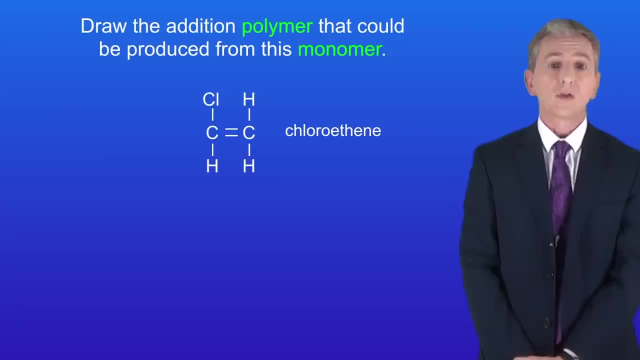 a question for you to try Draw the addition polymer that could be produced from this monomer. So pause the video and try this yourself. Okay, the monomer is chloroethene, so the polymer is polychloroethene and I'm showing that here Now you could be asked to draw the repeating unit.